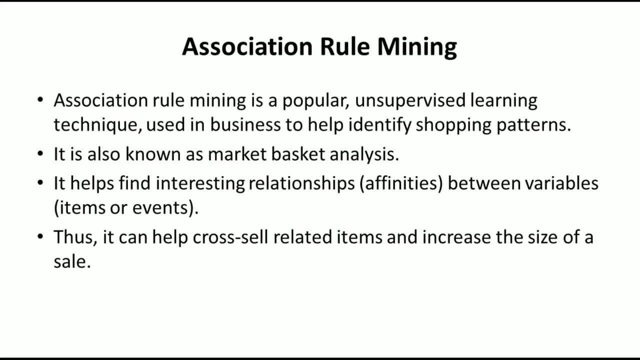 of that customer so that whenever he comes back- or can say that whenever a new customer came- We can facilitate the customer with those two products, because if he buys a product, there is a possibility that he will buy another product also. So that is what actually we. 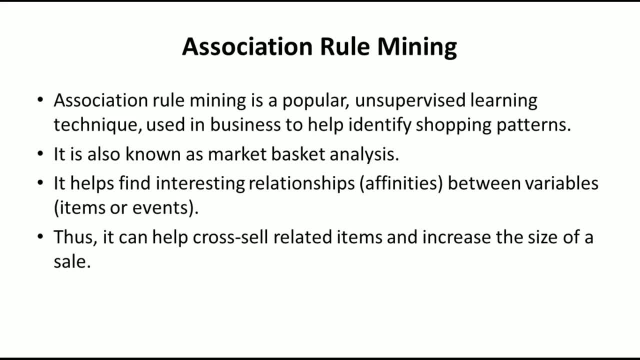 try to identify with the help of association rule mining. For example, if a particular person who buy bread and butter, he will also buy many times the milk also. So whenever you identify this particular pattern, so it is good for your business that whenever. 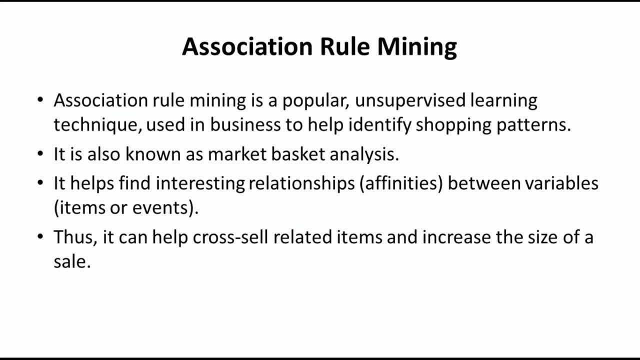 a new customer came, you can facilitate with all the three items in your shop so that you can use this particular cross, sell related items and increase the size of the sale. So that is what actually we can do. So this association rule mining helps in identifying the relationship. 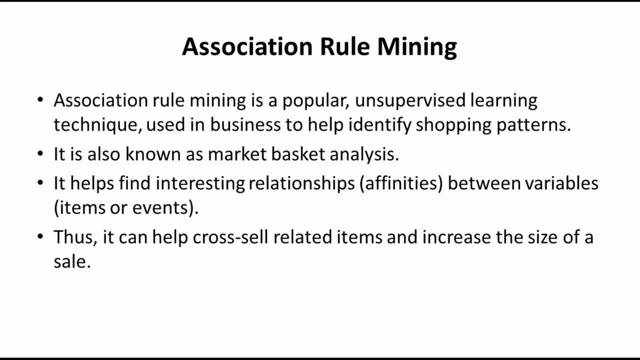 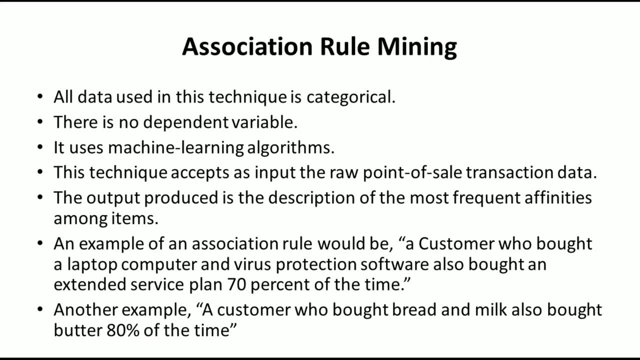 between the items and we can improve the sales size of that particular customer. So that is the main advantage of using association rule mining. Thank you, All the data in association rule mining is of categorical in nature. We don't use anything called as a continuous variable or numeric data. We use something called as categorical. 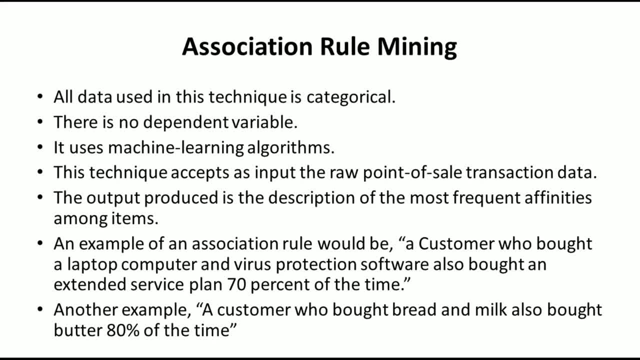 data In association rule mining. there is nothing called as dependent variable. Everything all the variables are called as independent variable. They are not dependent on one another. It uses machine learning techniques. Thank you, Thank you, Thank you. So the? so we will be taking the asset input as the raw point of sale transaction data. 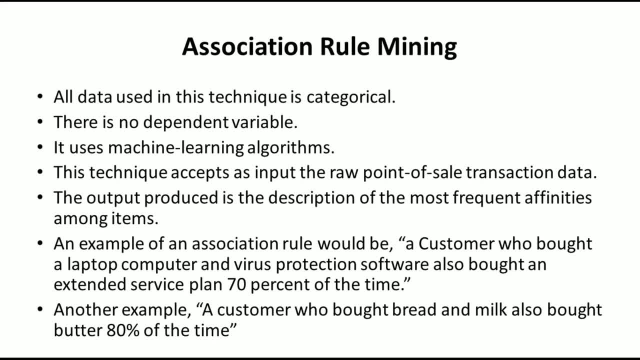 That is in a shop. we will be getting the point of sale data like who bought what product and so on, Starts the day off. who bought a laptop and a virus protection software. also bought an extended service plan of a service plan 70% of the time. so what is the meaning of this? one is a person who 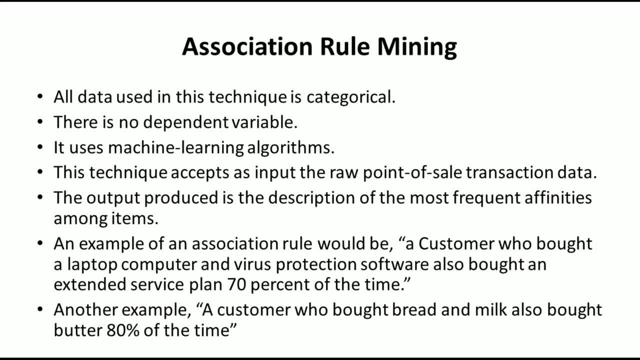 buy a laptop and virus protection software, he will be buying the extended service plan for 70% of the time. so whenever we try to sell we can say that the laptop and the virus protection, we can have something called as the extended service plan, also along with. 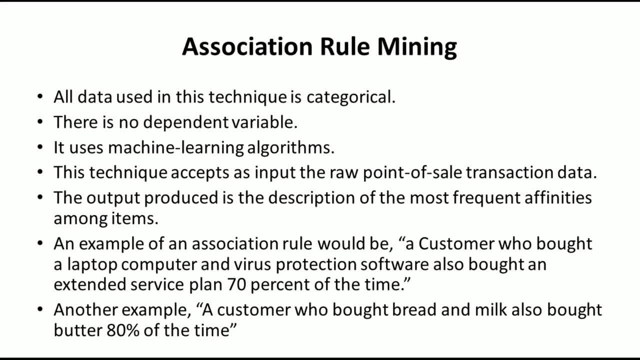 that, so that the next person will also buy it. so that is how we can improve or increase the sale size. another example is a customer who bought bread and milk also bought butter 80% of the time. so rather than having only bread and butter in the shop, we can have we. 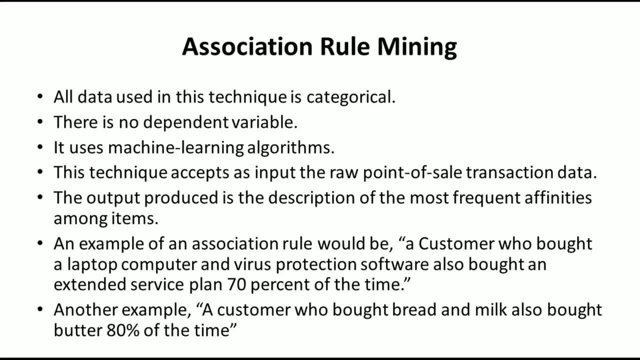 can say that better also. so, using this particular thing, what we can do is we can increase the sale size. the person who is buying two items will buy the third item also for 80% of the time. so understand this particular knowledge. we need to apply the association rule: mining. 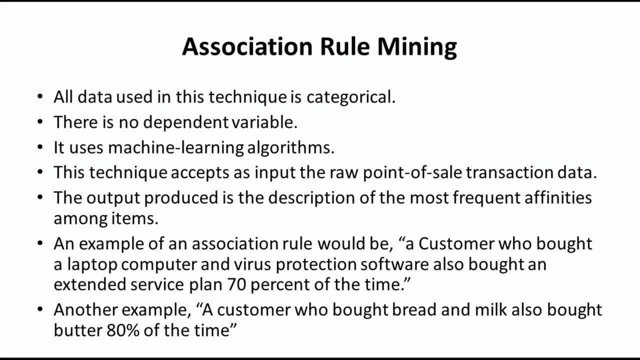 and then we need to get the relationship between the items, of the products which are present in the shop. once you get that particular, the relationship between the things, we can maintain the proper inventory in the shop so that we can increase the sales. so that's what the 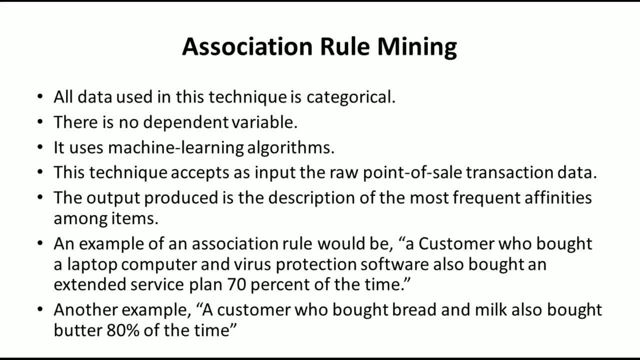 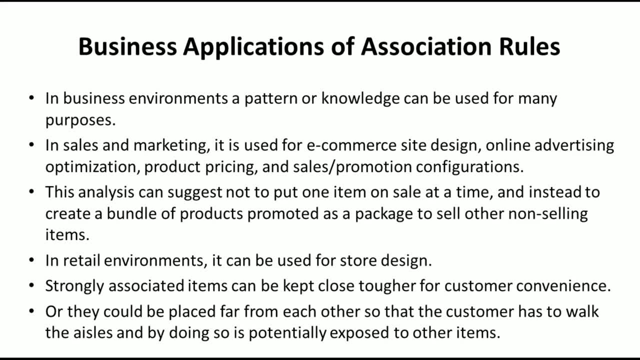 main idea behind association rule mining now where we can use association rule mining. so that's the next question: can I use it in X, Y, Z or application so on? that's what actually we need to understand In the online environment. patterns or the knowledge can be used for many purposes, whatever. 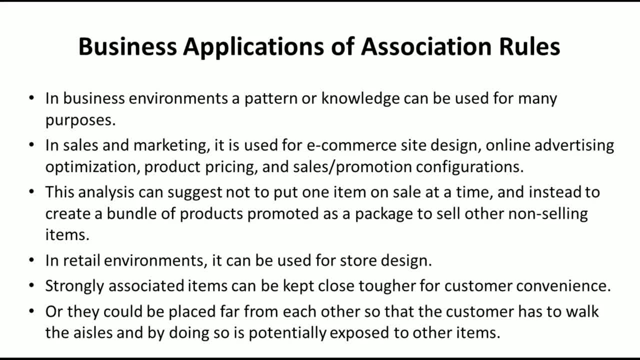 the knowledge we extract from the given data. we can use that particular thing for many purposes. in sales and marketing, it is used for e-commerce site design. when it comes to sales and marketing, it can be used in e-commerce site design, online advertising optimizations, product pricing, sales and promotion configurations. so in all these particular areas we can use. 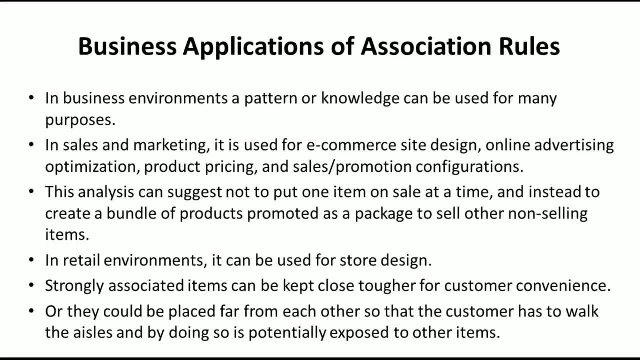 it So in e-commerce site design. So in e-commerce site design, For example, you go with any e-commerce websites like flipkart or amazon or something like that. whenever you try to buy one product along with that particular product, before you check out you will get some recommendations saying that a person who bought so and so product. 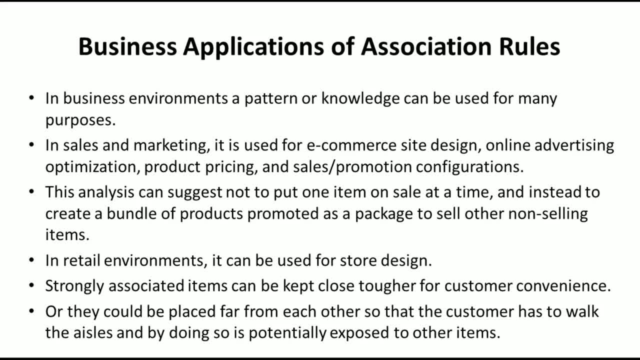 has bought these products also. so such kind of recommendations you get. so what is the meaning of that one is they have made, or can say that they have come up with, some association, association among the items? Whenever a person buy a particular item, They used to say that other persons have bought so and so item also. so that is what. 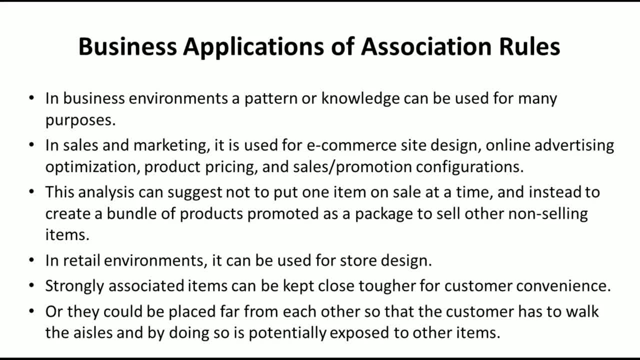 actually the use of association rule mining. The second one is something like online advertising optimizations. there is a possibility that a particular person is interested in certain kind of items. so rather than showing all kind of advertisement, what is to that particular person? we will show only the optimal advertise. 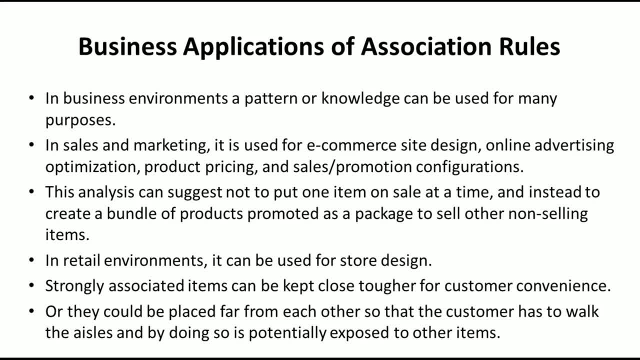 to those particular persons. So that can be done with the help of Association rule mining. now we can have the can set the product pricing, as well as sales and promotion configurations can be done with the help of for these algorithms. This analysis can suggest not to put one item on a sale at a time and instead create a bundle. 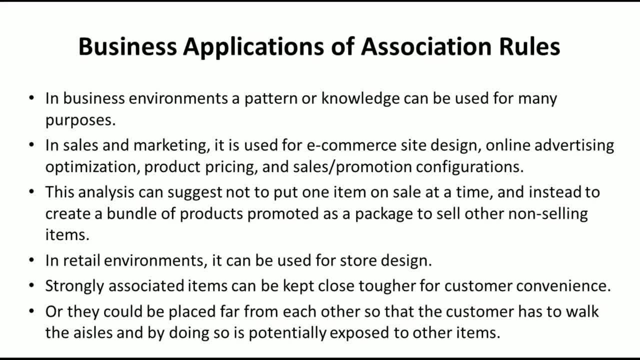 of products promoted as a package to sell other non selling items. so that's what the main advantage? rather than having one item in your shop, try to identify which item will be bought together And create a bundle of those particular products and try to sell them. so that's one advantage. 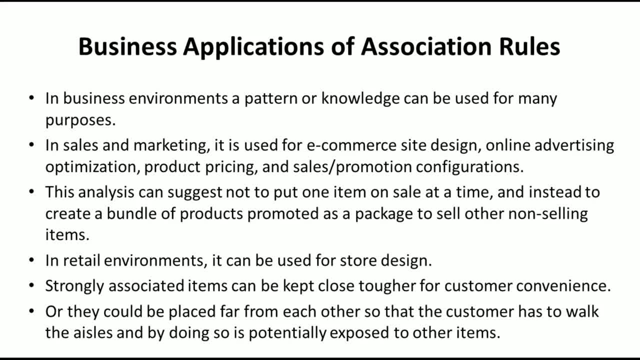 of the association rule mining In retail environments, or can say in the retail shops and all. we can use association rule mining for designing the store also. for example, let us say that there are two products which are bought together. what we can do is we can keep those particular products together whenever. 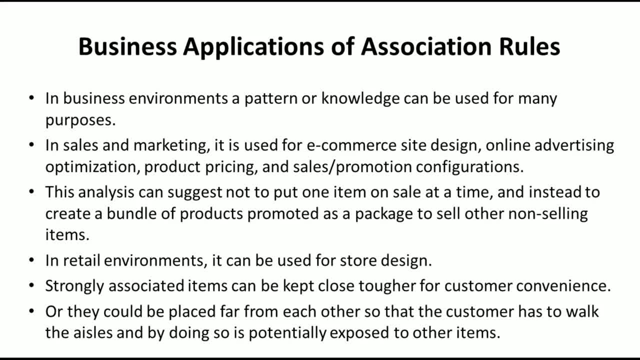 a customer comes and bought one product, he will see that another product is present next to it And He will buy that particular product. so that's the one possibility. there's another possibility, that the two products are bought all the time together. so what we can do is we can keep. 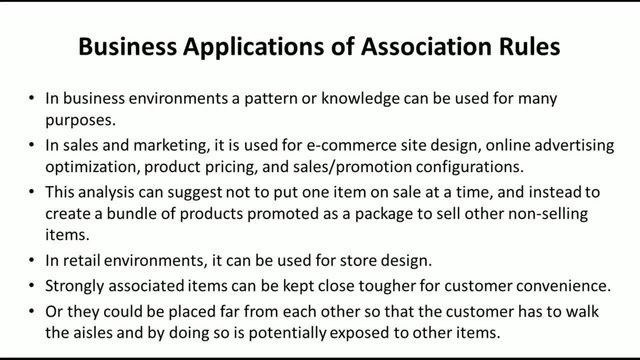 one product at one corner of the store and another product will be kept at another corner of the store. So what happens is whenever a particular customer comes to the shop, he will buy the first product, but he wants the another product, that's for sure. he will buy that second product because 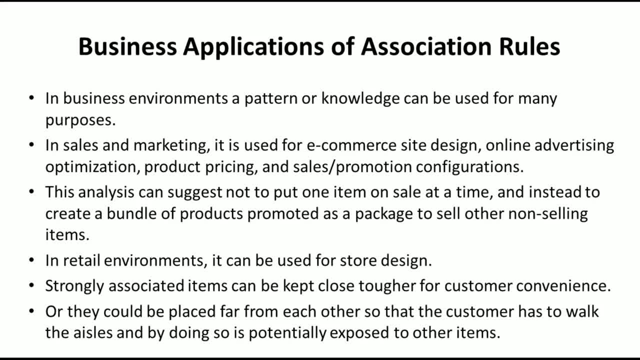 if there's only one product will not work over there, so he needs the second product. So what he does is he will search for the entire store for the second product. while searching he may come across with another products also, other products. he may buy other products also. 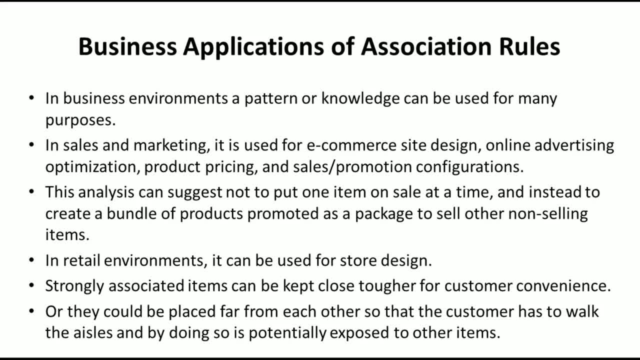 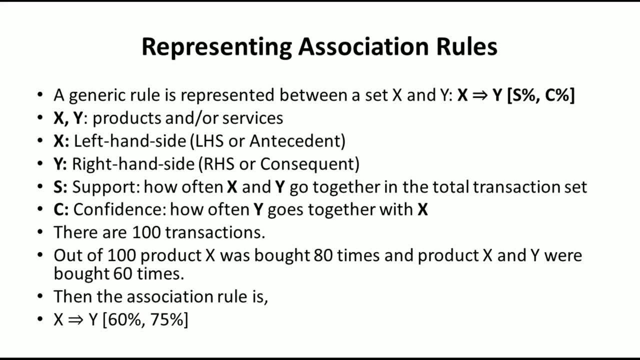 that is what actually: the way we can use the association rule mining for store design. Okay, So this is the how actually we can use association rule mining in different areas. Now, how we can represent association rule mining or association rules. that's all the very important thing. 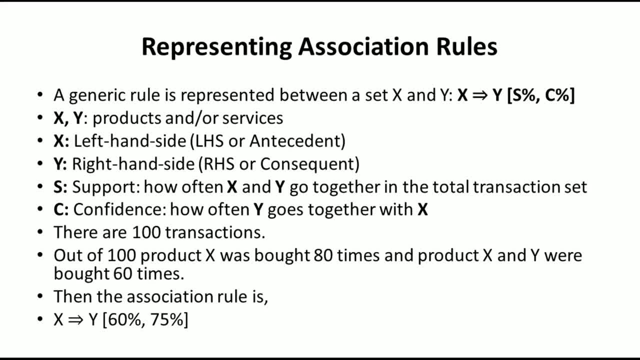 The generic rule is represented between the set of products. let us say that x and y are the two products. in this case the rule can be written something like: x tends to y, that is, x arrow y. x and y are the two products within square brackets or within curly braces. 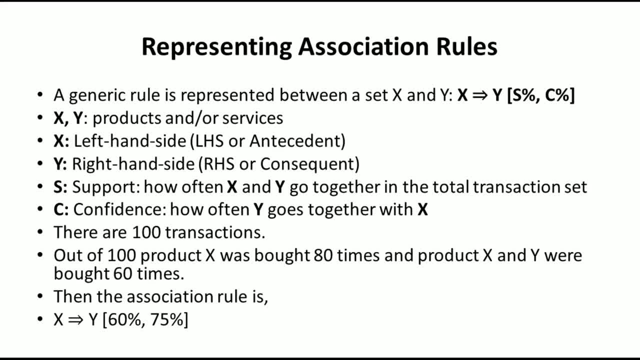 we can represent two variables or the two values. here one is called as support, another one is called as the confidence. Okay, so here x and y are the products, percentage yes or yes percent is the support and c percent is nothing But the confidence in this case. now, what is this? yes is a support. how can you calculate? 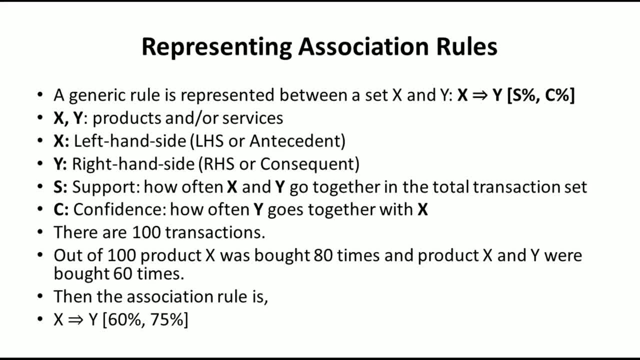 the support. that is, if you, if you consider x and y are the two products. we can calculate support like how open x and y go together in the total transaction set. So how often the items or the products x and y go together in a total transaction set that. 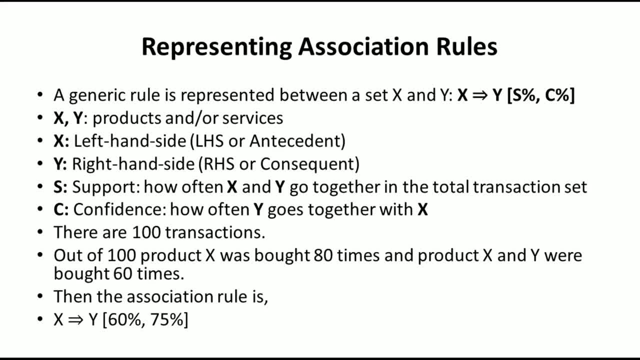 is nothing but a support. for example, assume that I will take first of all, what is the definition of confidence? So the confidence definition something like this: how often y, that is a product, y goes together with x? that is nothing but a confidence. So just take an example to understand these two definitions. there are hundred transactions. 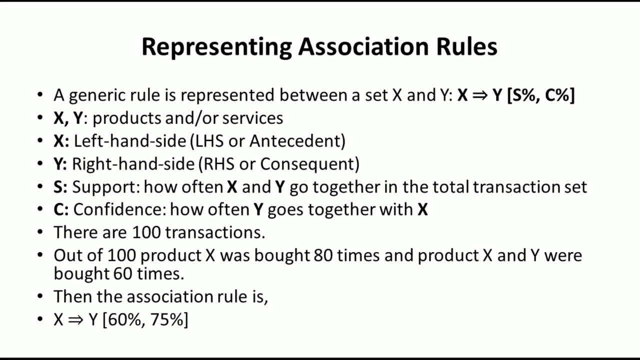 let us say that there are hundred transactions out of hundred transactions. the product x or the product x was bought 80 times and the product x and y were bought 60 times. So totally how many transactions we have here? There are hundred transactions we have out of hundred transactions. the product x was 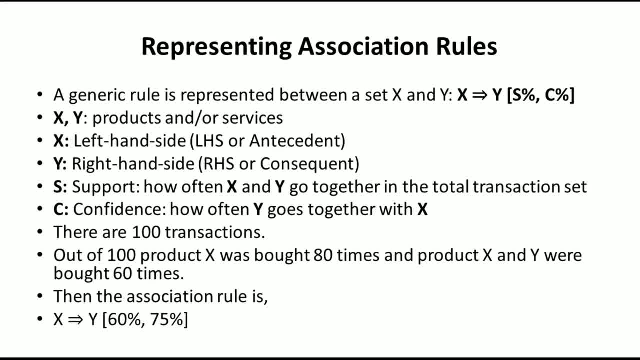 bought 80 times and the product x and y were bought together 60 times. this is very important. together, x and y bought together was 60 times. Now how can we calculate the support? support is nothing but what. how often product x and y go together in a total transaction set? that is the frequency of x- y, the divided by total. 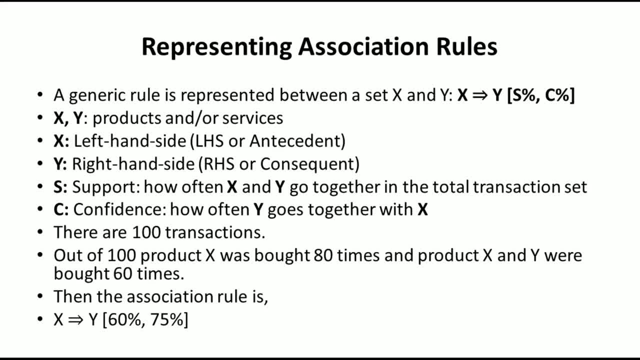 number of transactions. what is the frequency of x, y, 60 divided by total number of transactions, that is 100. so 60 divided by 100 is equal to 60 percent. that is nothing but a support in this case. what is the second one, confidence. how can you write, calculate the confidence? 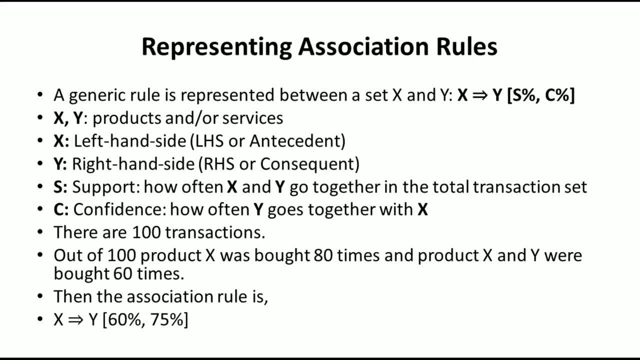 how often y goes together with x. so how often y and x and y were bought together 60 times? how many times x was bought 80 times? so 60 divided by 80, that is nothing but the confidence. In this case, that is equivalent to 75. if you want the equations, we can use these two equations. 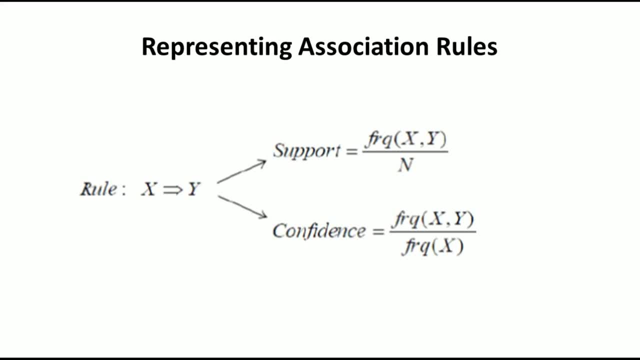 to calculate the support and confidence. in this case, the rule is: x tends to y. that is how often x and y were bought together. Now the support is equivalent to frequency of x- y divided by total number of transactions, that is n. confidence is equivalent to the frequency of x- y divided by frequency of x. 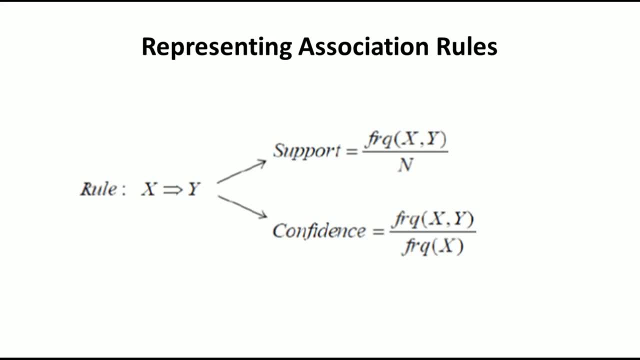 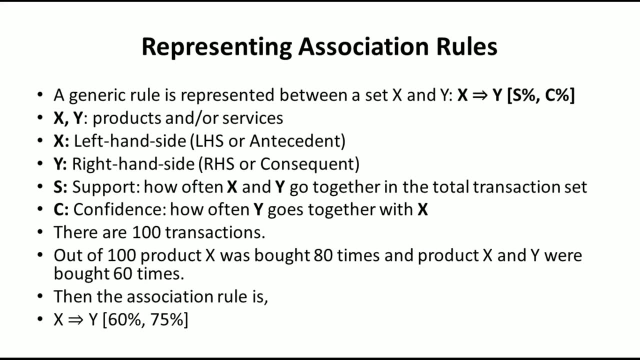 in this case. So this is how actually we can calculate the, The support and confidence. once you calculate the support and confidence, we can put those party things in either square bracket or curly braces to represent the affinity of the two products which are present in the association rule. 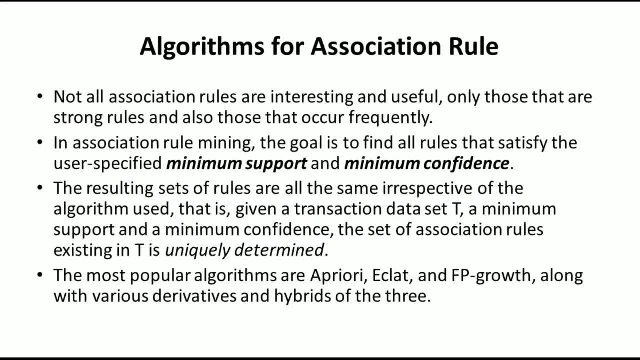 Now whether all association rules are useful. whatever the association rules we have written, whether all of them are useful. no, all of them are not useful or they may not have interesting features over there. Only some of those association rules are useful, those that occur frequently. you can say: 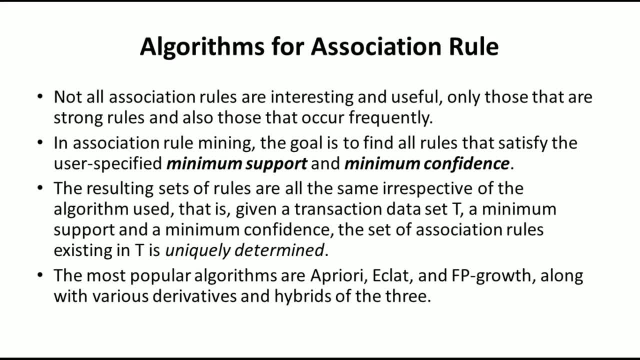 So the rules, which occurs frequently, they are useful. All the rules may not be useful for a particular retail shop or whatever the things. whatever the problem we are solving in association rule mining, The goal is the goal is to find all the rules that satisfy the users. specified minimum support. 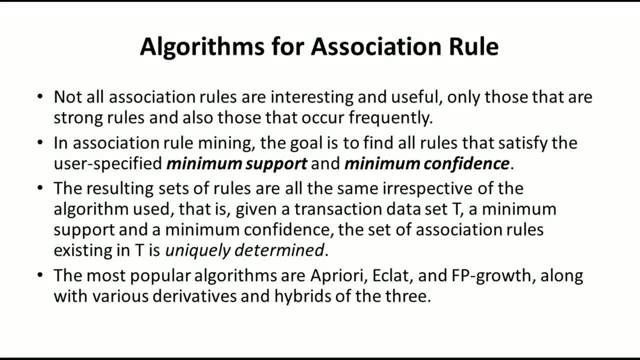 and minimum confidence. The user must have some confidence in that, must have specified the minimum support and minimum confidence. we need to find all those rules which satisfy this, these two requirement, that is, the minimum support as well as minimum confidence. so what I supposed to do is I need to write all the rules. I need to find what 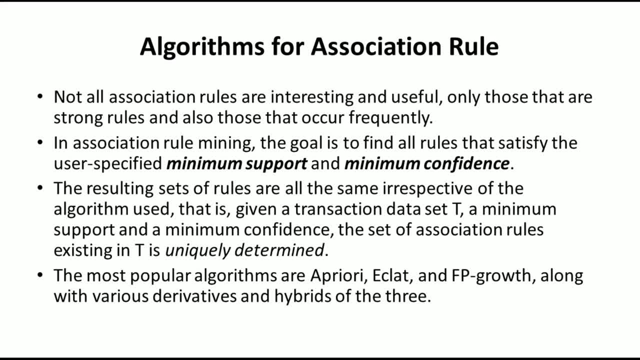 is the support and confidence of that particular rule, and later I need to check whether it satisfies the minimum support as well as minimum confidence. if it satisfies the minimum support and confidence, the meaning of that is that rule is useful for your organization or it may not be useful for your organization or the problem under consideration. the resulting 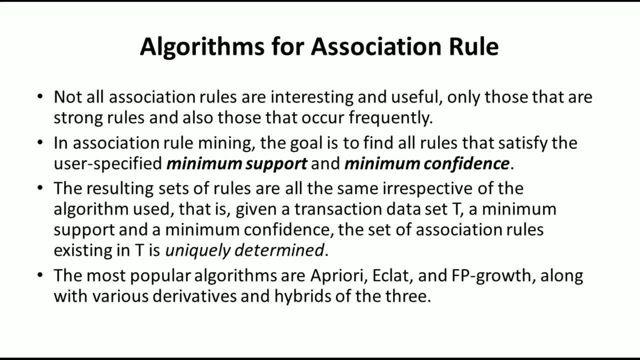 set of rules are all the same, irrespective of the algorithm used. that is, given the transaction data set T a minimum support and minimum confidence, the set of association rules existing in T is uniquely determined. one of the most popular algorithm for association rule mining is Apriori. 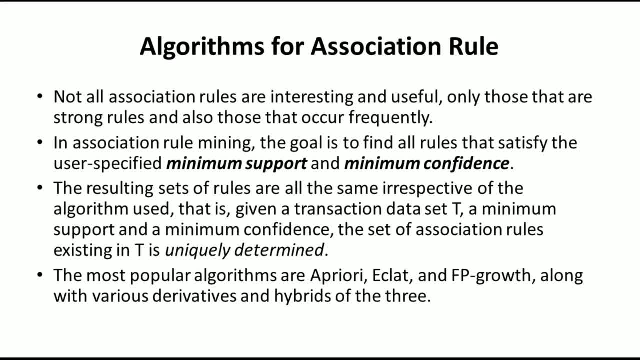 the other one is Ecclate, The third one is Scalpel, The fourth one is something called as FP growth, all with various derivatives and hybrids of three. in this video I will be discussing Apriori algorithm and remaining algorithm I will discuss in other videos. the link for the same can be found in the description below. 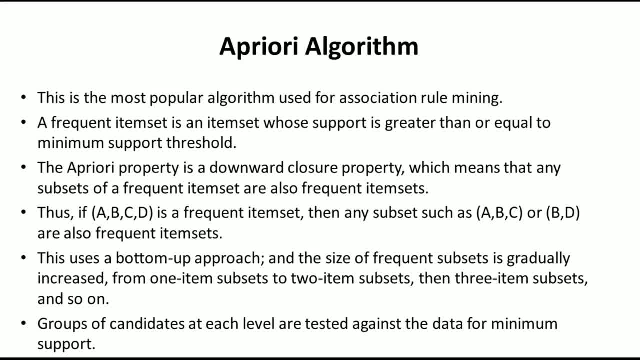 Now how Apriori algorithm works. so that's the first question we try to understand. this is the most popular association rule mining algorithm used for identifying the frequent item set. a frequent item set is an item set whose support is greater than or equal to minimum support threshold. what is frequent item set? that's the main question we need. 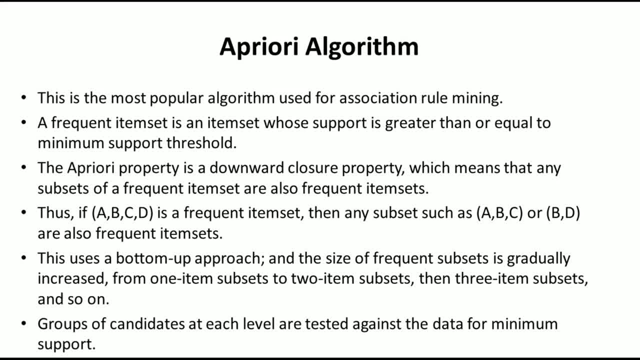 to understand here what is the frequent item set? and a frequent item set is item set. it is not something different. it's item set but whose support is greater than equal to minimum threshold value. so the user must have set some minimum threshold value. if the support of the item set is greater than the minimum threshold value, it will be called as the frequent. 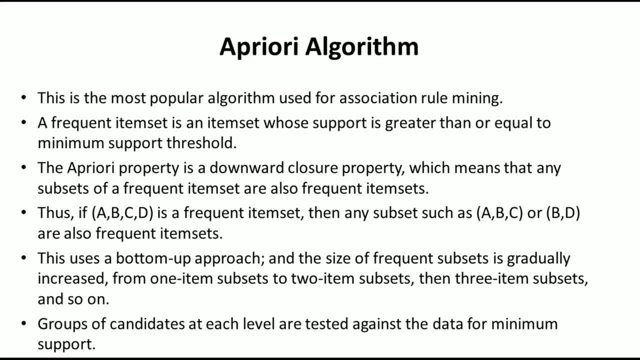 item set. the one very important characteristics of a frequent item set is that the frequent item sets are downward closure, have a downward closure property. what is the meaning of this? for example, if ABCD is an frequent item set, then any subset of ABCD is also a frequent. 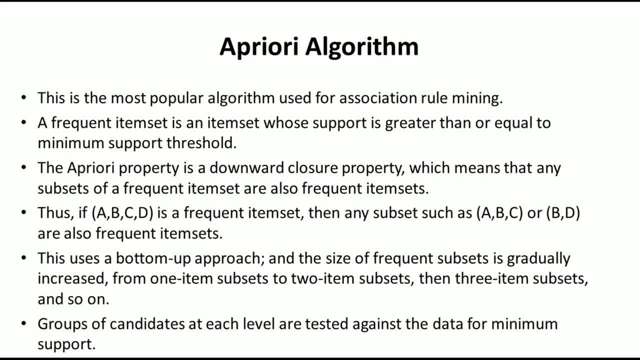 item set any subset. when I say it is, it's a- any non empty subset. for example, if you have ABCD as the item frequent item set its subsets A or B. the third item set is frequent subset is C or fourth one is D or AB or AC or AD, ABC, ACD, ABD or BCD, everything every. 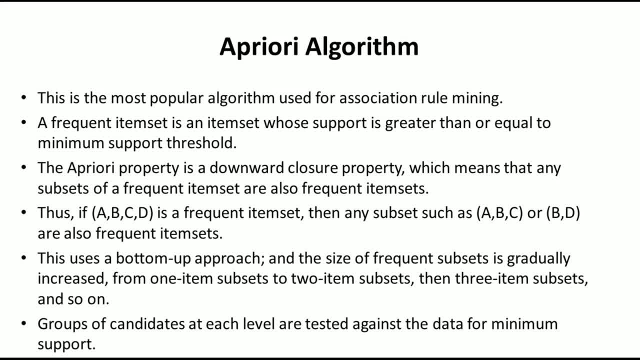 every subset is also a frequent item set. the Apriori algorithm uses bottom-up approach. that is the first. it'll 32.3, two words, the frequent item set, starting from one item set at a time. so initially it will consider one item set and then it will calculate whether these one item sets. 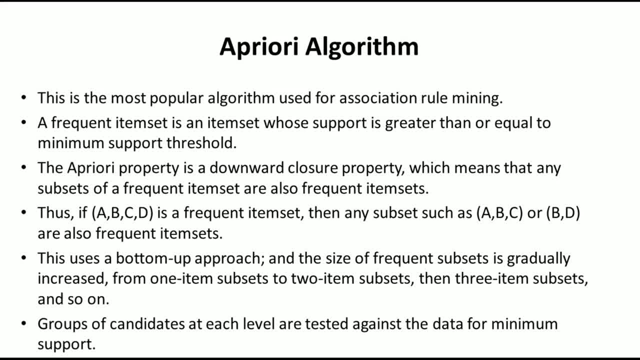 are a frequent item sets or not, that is, whether they satisfy the minimum support or not. after that it will increase it to two item sets at a time. once it calculates the two item sets, it will calculate whether those things are two frequent item sets or not, and then it will be increased to three and so on. so 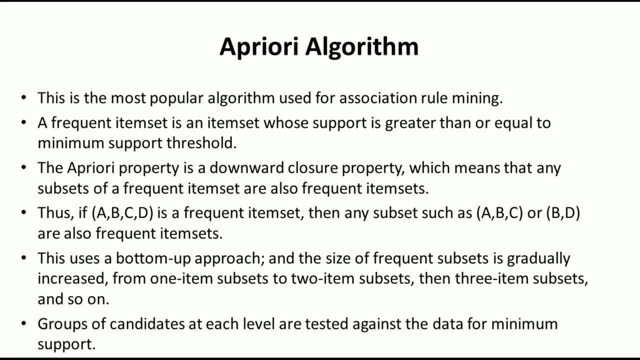 that's how actually it works. so we will take one very simple example to understand that property at the later stage. once you calculate the frequent item sets, the next thing is to calculate the. you can say that the items or the we need to write the association rules by considering the confidence. so one way. 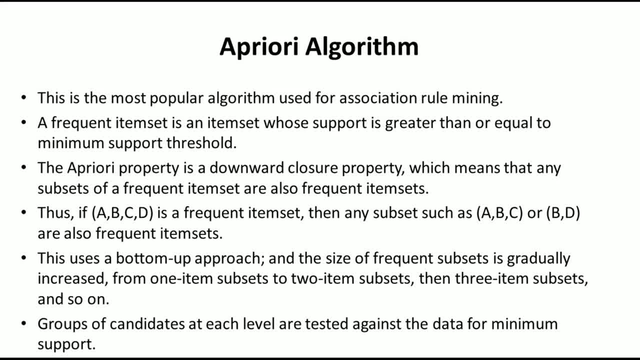 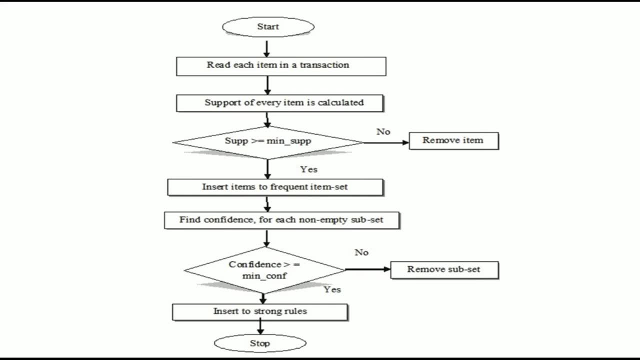 the rule which satisfy the confidence. the meaning of that one is that particular rule is useful for your organization or a problem under consideration. so this is how I actually the flowchart of the up-rear algorithm looks like. as I told you earlier, it has two parts. first, we need to calculate all the frequent item sets. the second part: 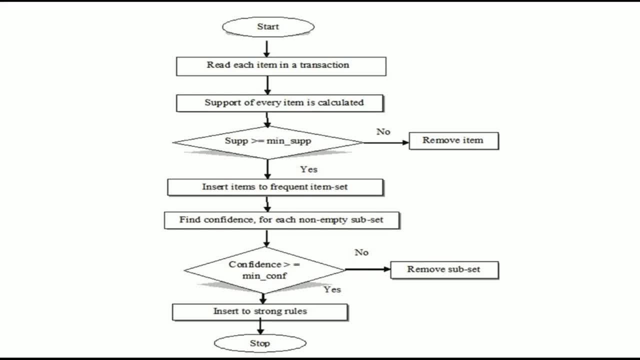 we need to calculate the association rule, mining association rules actually, which will satisfy the confidence. okay, so that is how actually it works. so initially we start with each item in a transaction- okay, one item at a transaction- and then we set for example, for example, we which whether a particular item has a sufficient support level or not. if it has a sufficient support level. 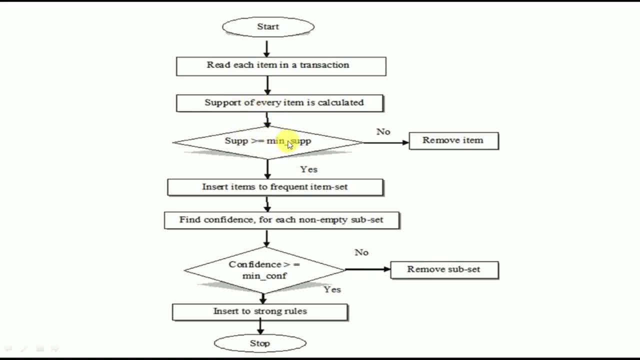 or you can say that the support of that item is greater than the minimum support. we'll insert that particular thing into the frequent item set, otherwise we remove it. okay, so once it is done, we go back and then what we do is we will consider two items at a time. we check whether the support 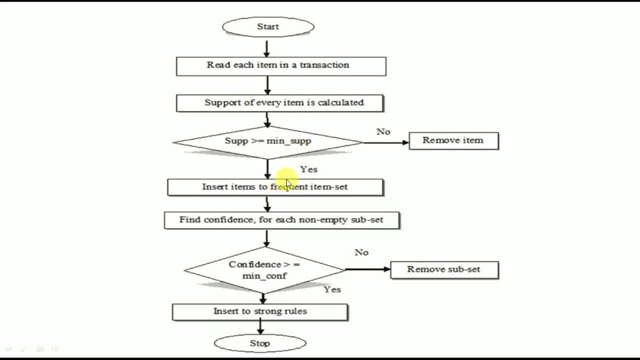 is greater than or equal to minimum support. if yes, include those things into frequent item sets. otherwise, remove that particular frequent items item sets. the same thing will be repeated, for you can say that all possible combinations of items. once you get all the frequent item sets, the next thing is to reduce or write the rules of that particular thing. so how to write the rules? 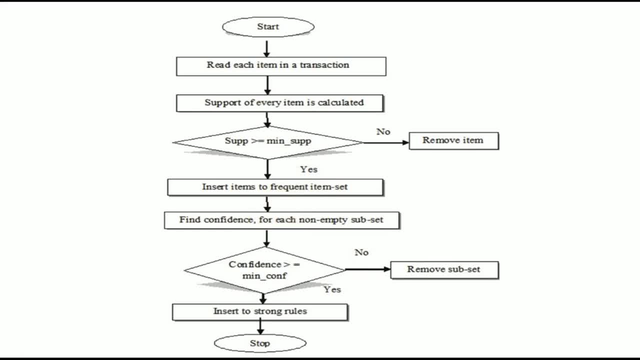 we need to write the association rules. once you write the association rule, we need to find the confidence of that particular association rule. if the confidence is greater than the minimum confidence, the meaning of this one is that's a strong rule which is useful for your organization or the problem under consideration. 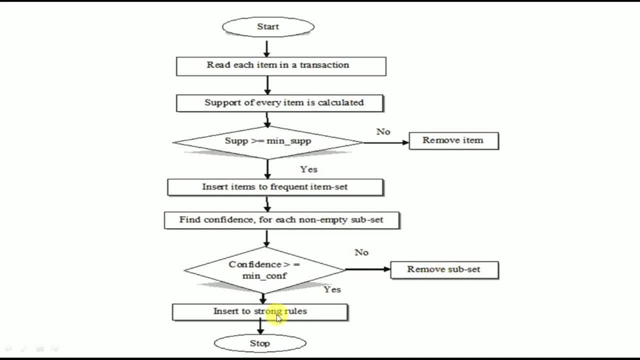 otherwise we need to remove that particular rule. the same thing has to be repeated for all the frequent item sets and we need to identify all the rules which are strong rules. you can say the. the rules are called a strong, strong rules if the confidence of that rule is greater than. 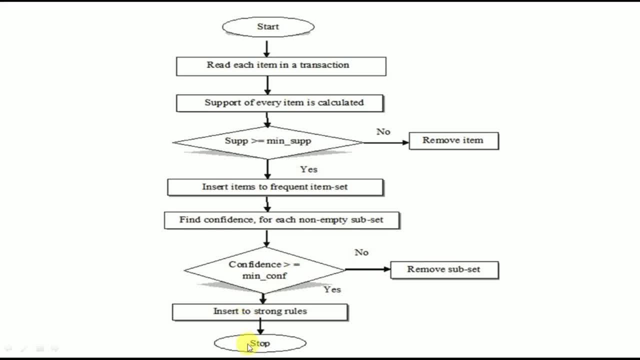 the minimum confidence greater than equal to minimum confidence. so once everything is done, we can stop the algorithm. so in this video, what i have done is i have given a brief introduction to association rule mining, as well as i have introduced what is a prior algorithm. the next, 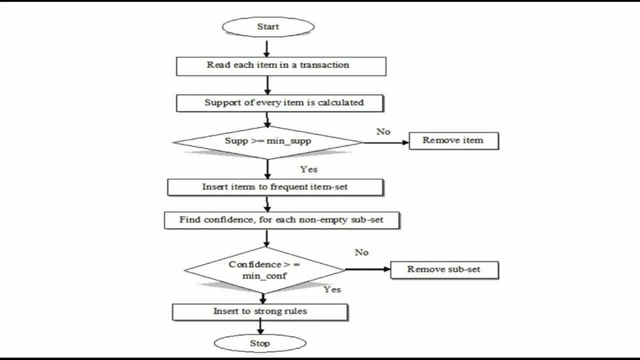 video i will be discussing how can we solve what numeric can say that the upper algorithm. considering one very simple numerical example, and later i will discuss how to implement this upper algorithm in- we can say that different programming languages like python are, as well as like microsoft, excel and weka. okay, the the link for all those videos are given in the description. 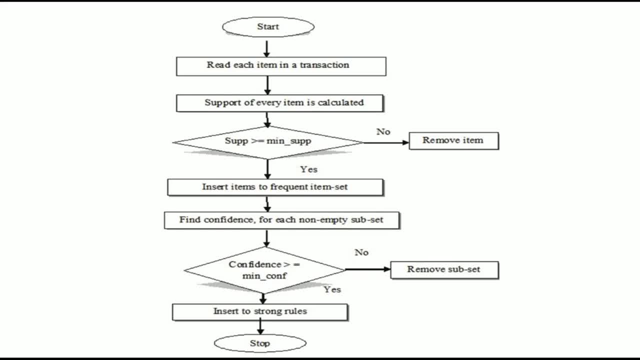 below. if you want, you can watch this particular videos. i hope the concept is quite clear. if you like the video, do like and share with your friends. uh, press the subscribe button for more videos. press the bell icon for regular updates. thank you for watching.